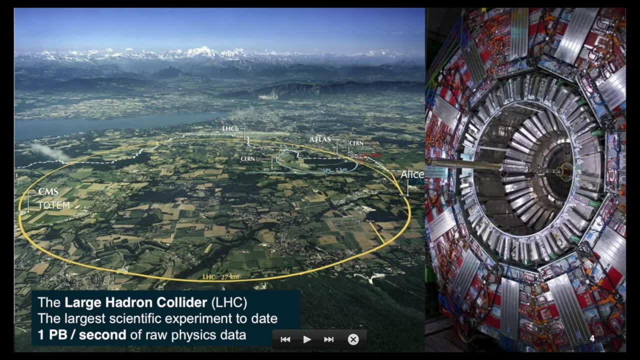 the LHC, the Large Hadron Collider. The LHC is a particle accelerator. It's actually the most powerful particle accelerator in the world. It's actually built, as you see here in this picture, in the Franco-Swiss border, So you have there Lake Geneva and the Alps. 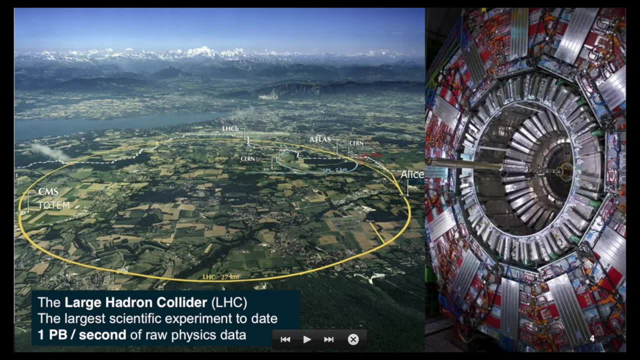 And it's built in a tunnel that is 27 kilometers long. And inside this tunnel, inside this ring, what we do is we accelerate particles close to the speed of light And then we make them collide against each other And we observe what happened in those collisions. 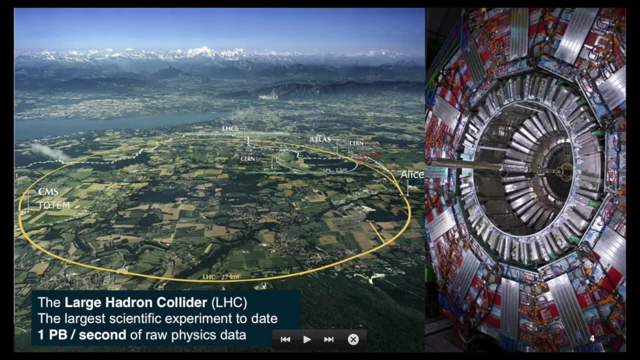 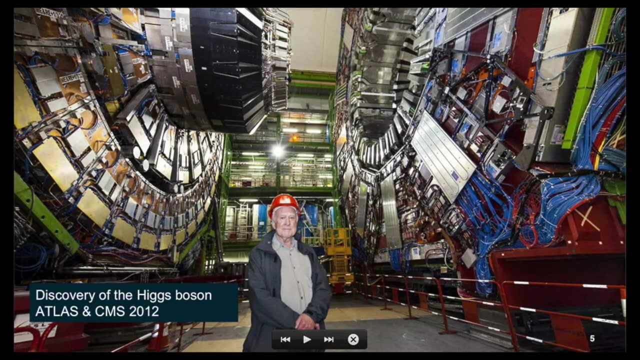 So actually, the collisions, they happen in particular points of this ring, which is what you see on the right of this image. These are called detectors And they have all these layers of sensors that will capture what happened in the collisions in the LHC. 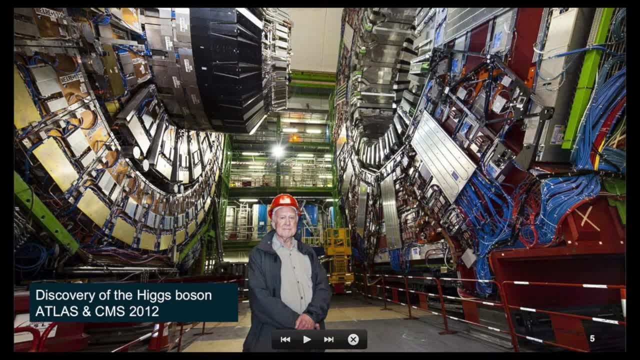 So the LHC has led to several discoveries. Perhaps the most famous one is the discovery of the Higgs boson in 2012.. Actually, you see here in the picture Peter Higgs, who, together with Professor Engler, They actually predicted the existence of this particle in the 1960s already, but only was. 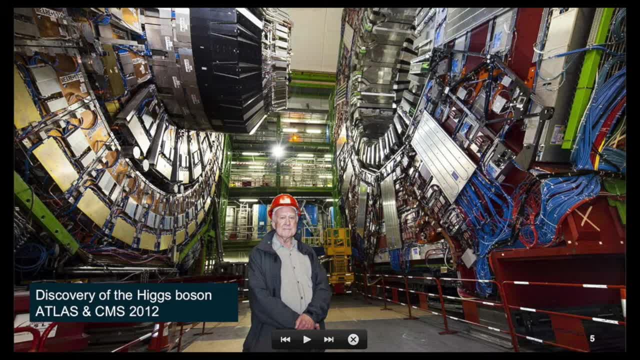 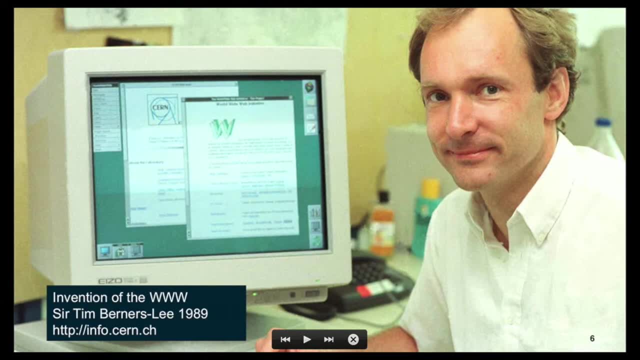 demonstrated empirically by the LHC in 2012.. But particle physics aside, CERN was also the birthplace of the World Wide Web. So actually, the web was invented by this man in the picture, Tim Berners-Lee, when he was. 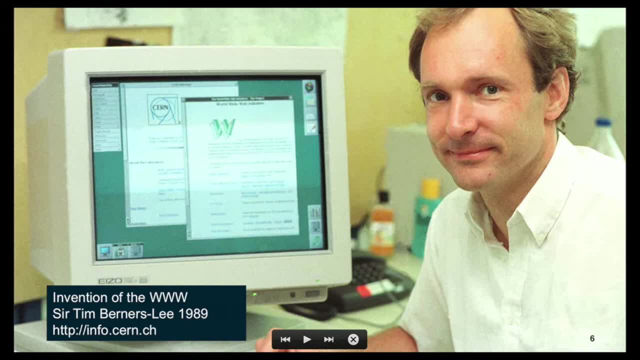 working at CERN in 1989. So he basically needed some way to share information with his colleagues. So he put up this next server, the first web server ever, at this URL infocernch. And actually, if you are curious, you can still go to this URL and you will see the. 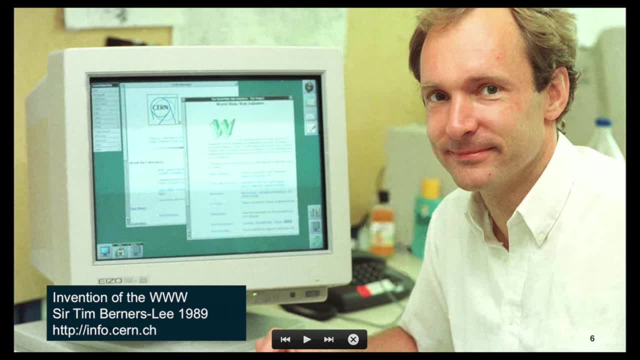 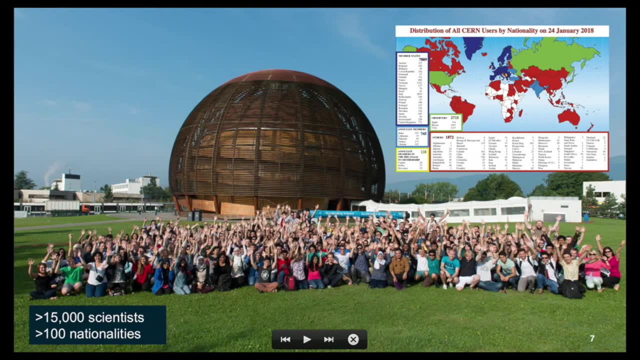 first website ever that Tim Berners-Lee created which was hosted at CERN. So at CERN we are a very international crowd. We are more than 15,000 scientists, Some of them work at CERN. they are raised at CERN. 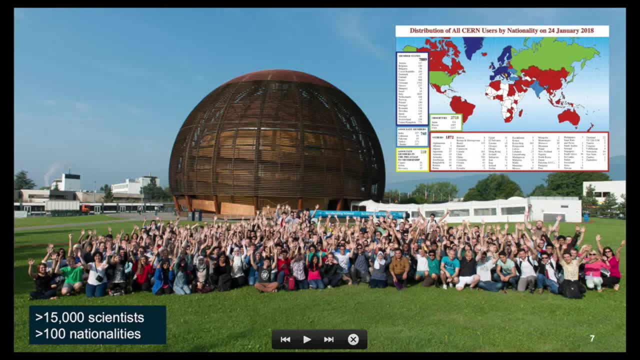 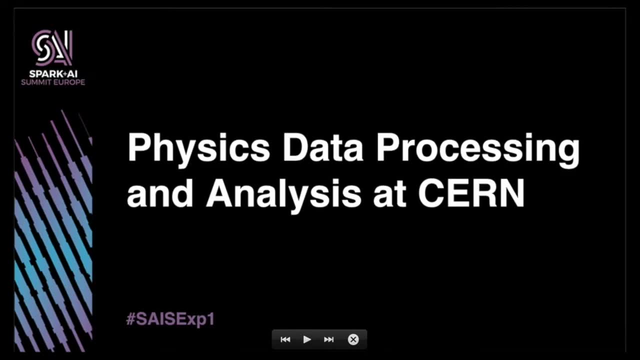 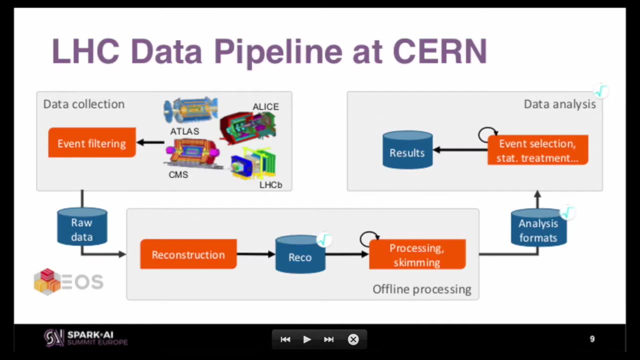 Some of them they work in other institutions collaborating with CERN, And we come from more than 100 nationalities. So how do we actually do data processing and analysis at CERN? This slide actually summarizes how we do it. It's the whole pipeline that data follows at CERN. 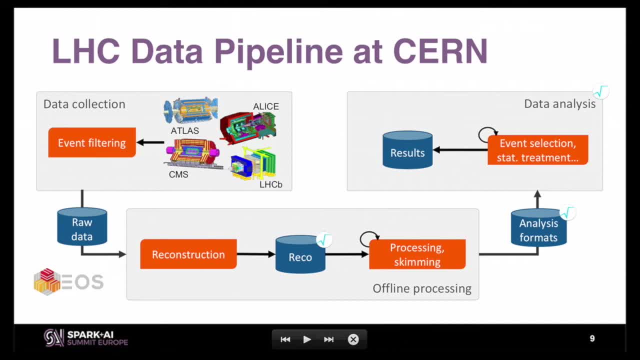 So we start with the detectors, so where the collisions happen, This generates a lot of data. this generates actually one petabyte per second of raw data, But of course this data needs to be filtered. So we do a process of filtering this data by hardware, with FPGAs, and software, with some. 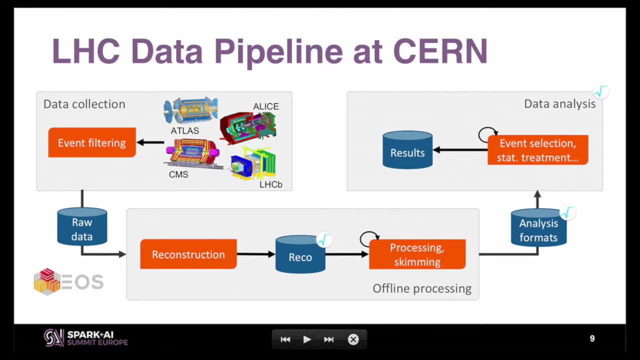 physics algorithms, And then we are left with one petabyte a day of data. So from one petabyte a second to one petabyte a day that we actually store in our mass storage system that is called EOS. So this is raw physics data. 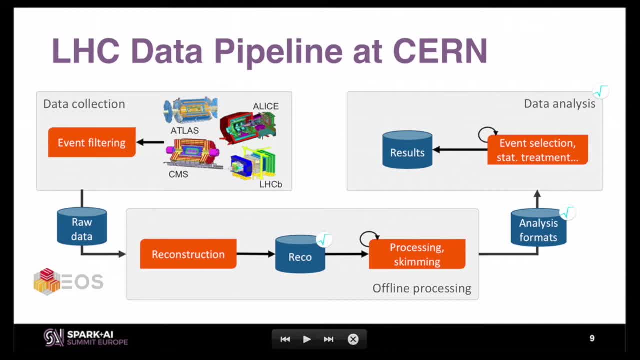 Raw collision data That then we need to reconstruct. So reconstructing means that we need to find out what were the particles that came out of this collision And we need to know what were the trajectories, the tracks that they followed, So that we know exactly, we have a complete picture of each of the collisions. 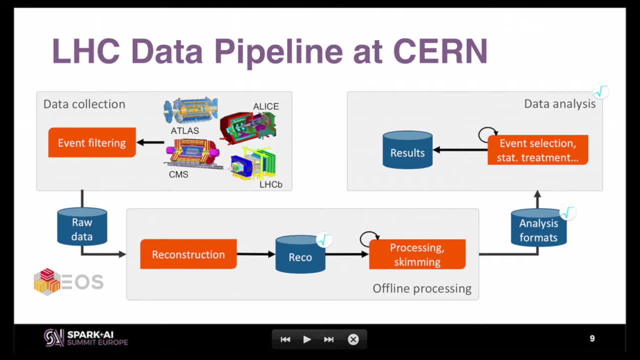 So we do this reconstruction. we generate the reconstructed data, which is already in root format- I will explain in a minute what root is- And then this data goes through further processing and skimming that results in some analysis formats, which is actually what the physicists will use to do their final data analysis. and 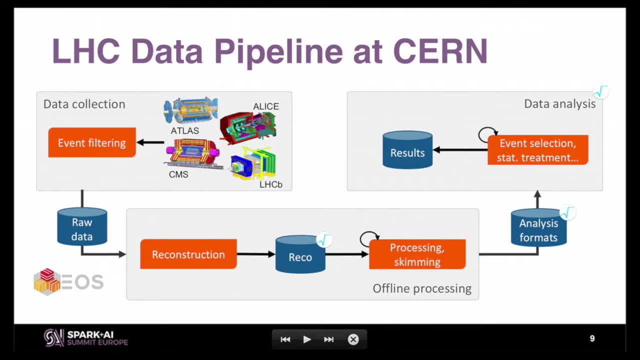 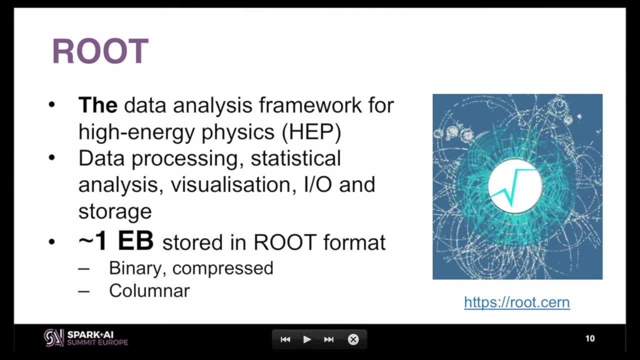 get physics results. So this is a whole picture of how data flows at CERN And how do physicists analyze this data. So they basically what they do is they use this data analysis framework that is called root, Which is widely used in high energy physics. 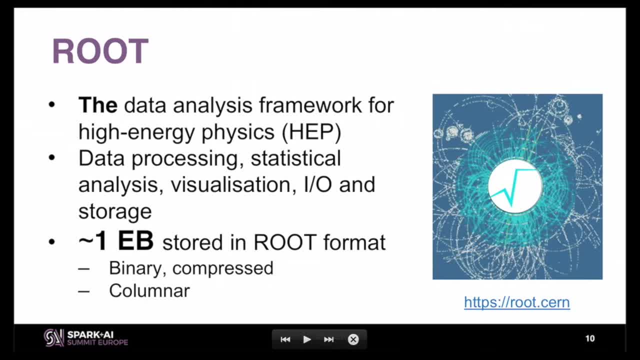 It's a software toolkit that you can use to do data processing, statistical analysis, visualization, IO and storage of data, And actually now we are close to one exabyte of data that is stored in root format- Data coming out from the LHC all over these years since the creation of the LHC. 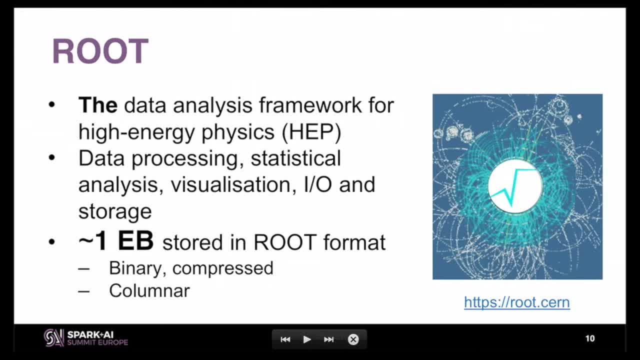 Now we are close to this one exabyte And this root format is actually. it's a binary format compressed, and it allows physicists to store data in a columnar format, Data in a columnar layout that looks a little bit like this: 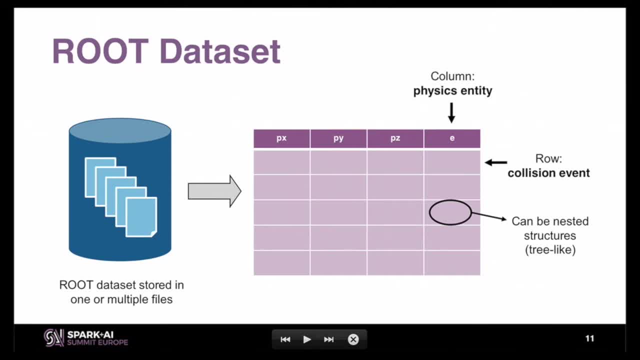 So this is a typical root data set. It can be stored in one or more files And it has this layout where the rows are the collisions, the collision events, And the columns they are physics entities or physics quantities that are related to that particular collision event. 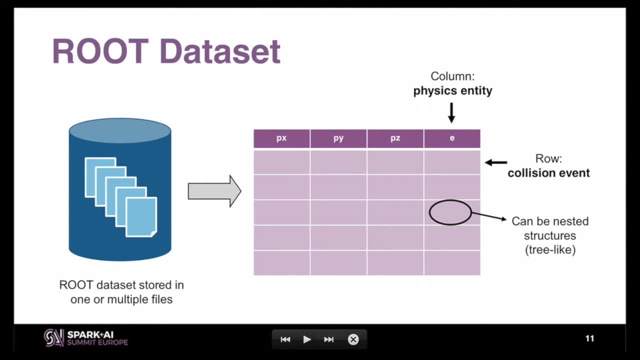 And actually the collision events. they are independent between them, So you can just process them in parallel, No problem. They are stochastically independent And, although this looks like a table, actually each of these physics entities. they can be complex C++ objects like an electron or muon. 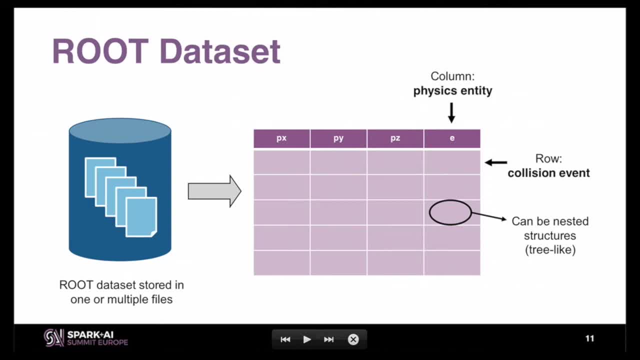 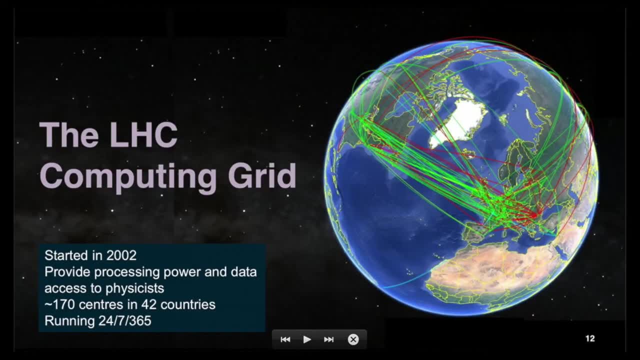 So it's actually more a nested structure that looks more like a tree more than like a table that is shown here. So in order to process all the data that was coming out from the LHC, CERN initiated the creation of the LHC computing grid. 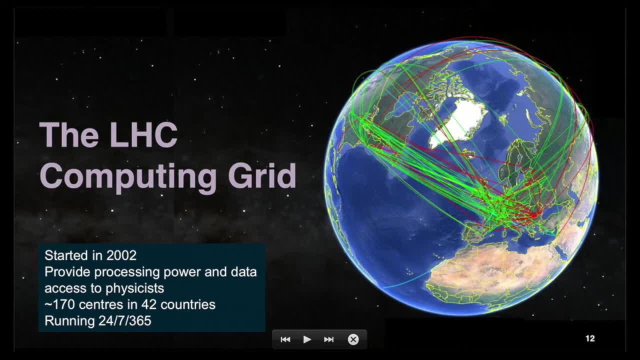 So it started in 2002.. And it's basically used by physicists to submit their jobs and process their data. It's formed by many computer centers all over the world that contribute with their resources in terms of storage and processing resources, computing resources. 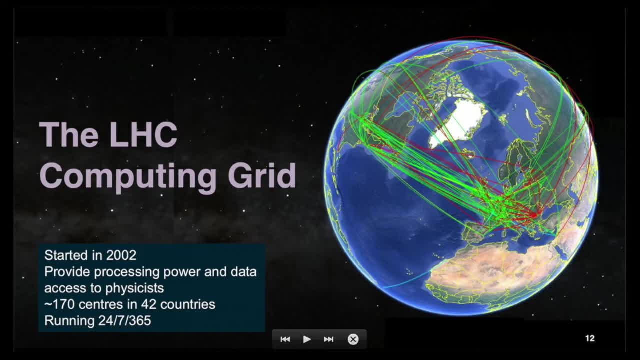 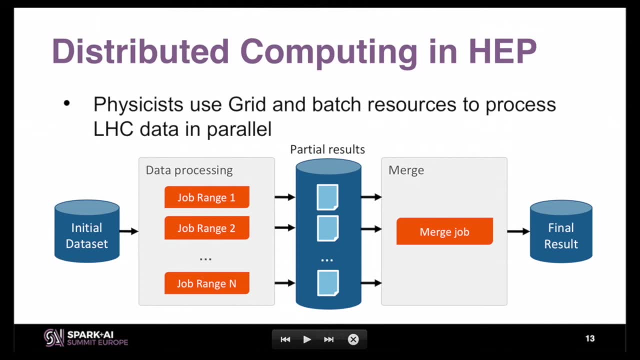 And it's running 24-7, all year long. So this is actually what the physicists used to do: Run their computations, And the typical workflow that they follow is they have some data set that they want to process, So they take this data set and they create ranges. 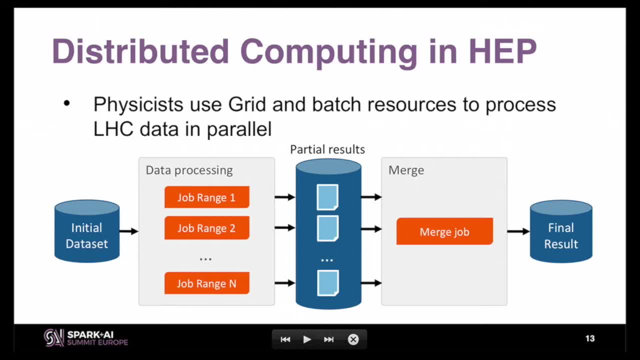 And for each of these ranges of events. so these are collision events. they launch a job in the grid, A job will process a range, Then these jobs, they write some partial results And then there will be afterwards a merge job that will merge these partial results. 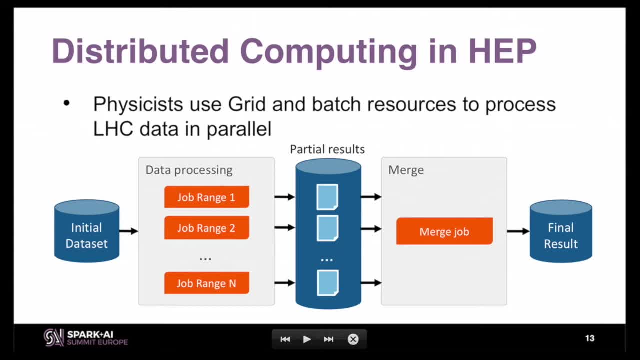 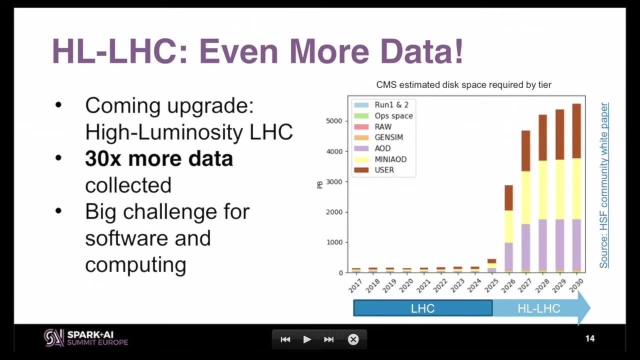 So this is typically how it works, how physicists work. This is a model that has been used over the years and has allowed to analyze tons of data, But there are huge challenges that are coming ahead. So in a few years, we will have this very important upgrade of the LHC, which is called 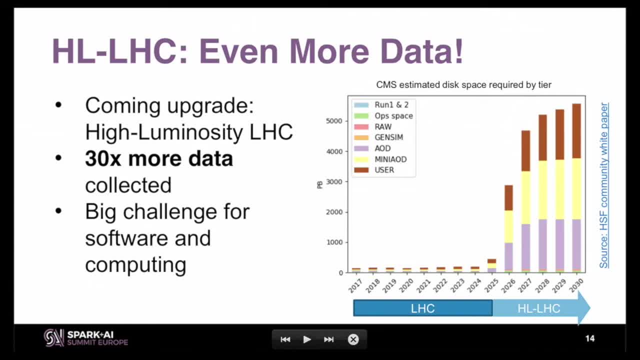 HL-LHC or high luminosity LHC. High luminosity basically means more collisions, And more collisions means more data. So we estimate that we will collect 30 times more data than the exabyte that we have already collected in this HL-LHC period. 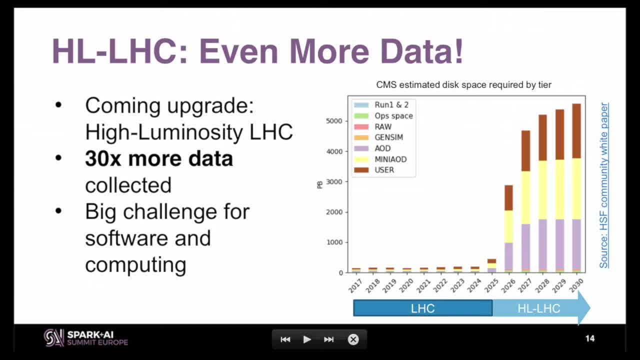 So it's a huge increase And this poses a big challenge for software and computing, because if we see the estimated technology evolution until that year- until 2025, and the data processing needs that we will have, then it's clear that software needs to bridge this gap. 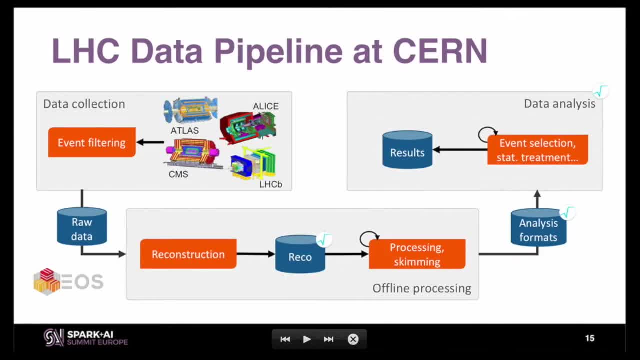 Okay, So we are working on that And actually I showed this already. this is data pipeline and all the stages in this pipeline at CERN. they will all be pushed by this data increase, All of them, But in this presentation I will focus on one of them, which is the final data analysis. 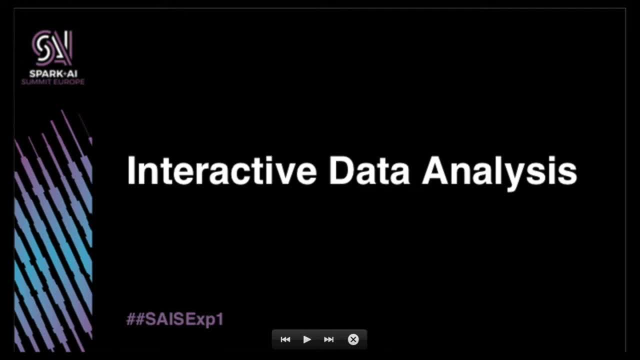 that physicists do. So in that sense, I wanted to introduce to you this interactive data analysis platform, and I'm going to show you how to do that. So let's get started. So this is the data analysis platform that we have set up at CERN. 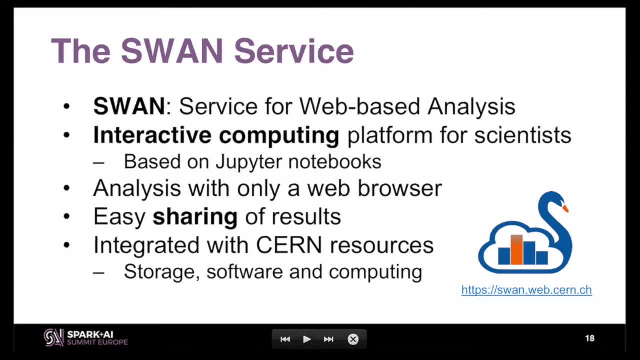 And this platform is actually called SWAN, the SWAN service, So it's a service for web-based analysis. The idea is that with this service, people connect to it, they authenticate with their CERN credentials, with their browser, and they get an interactive computing interface. 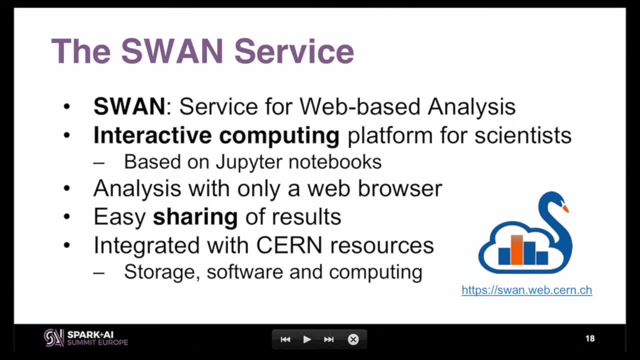 based on Jupyter notebooks where they can run their analysis. Okay, So this is the data analysis platform. It also allows- and we will see it in a minute- easy sharing of results So you can do collaborative analysis. You can produce your notebooks and share it easily with others. 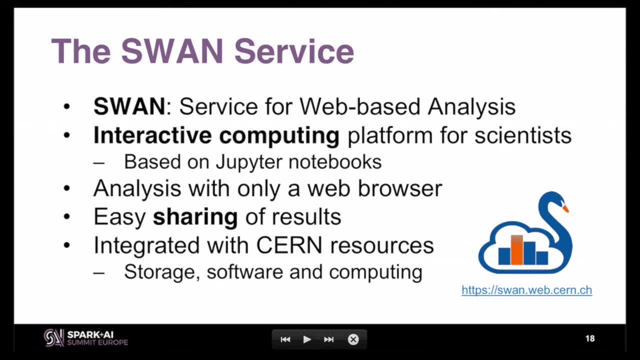 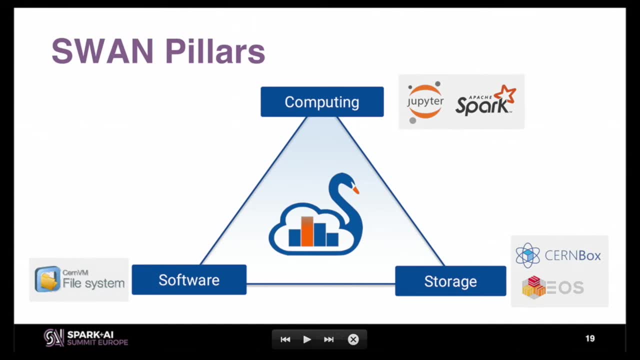 And it's integrated with the whole ecosystem of CERN resources, with technologies that are already familiar to physicists at CERN, that they use every day for their work, And I'm talking about technologies in terms of software, storage and computing. So any service like this. 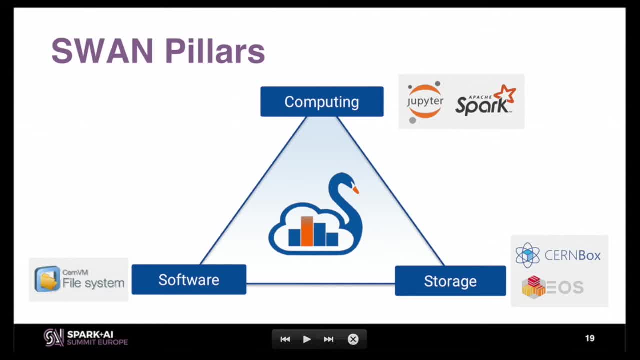 Okay, To start with software. any service like this needs to provide the software that physicists or that users in general need, because otherwise they will not use it right. So for that our choice was very clear: We provide access in this service to CBMFS, which is a distributed file system that we 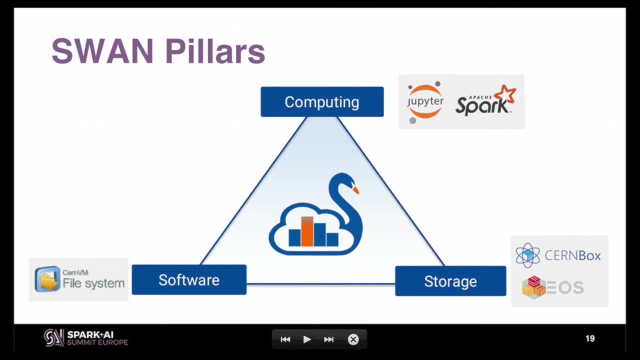 have at CERN, where all the experiment software, all the physics packages that our scientists need, they are there installed so they can use them from SWAN. Okay, Then, another important pillar is storage. A service like this needs to provide access to data, otherwise users will not use it. 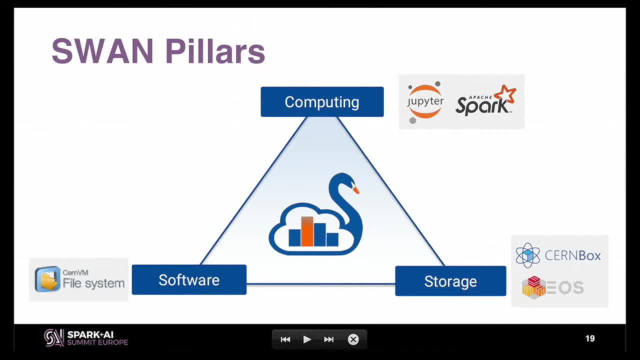 They need to find the data that they want to use And for that we make accessible the data on this EOS mass storage system that we have at CERN, So all the LHC data is put there. So we need to make it accessible. 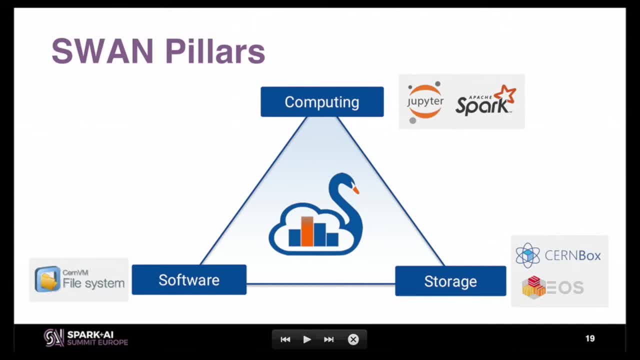 And also we have this sync and share part which is called CERN box. It's a little bit like Dropbox at CERN, which is just user files- Okay, It's user accounts with some user files that they also want to have accessible. 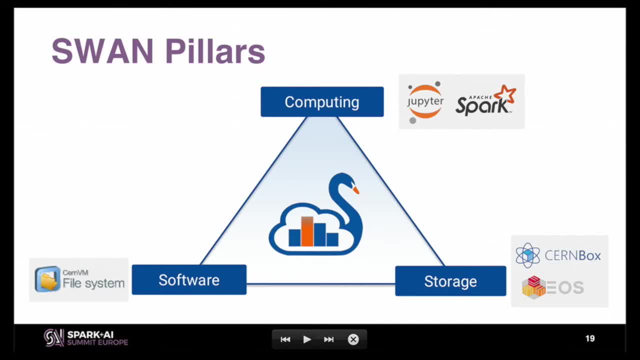 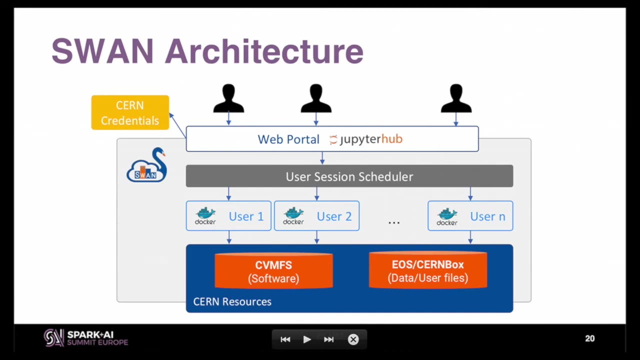 And then finally, computing. We do it with these interface Jupyter notebooks and with Apache Spark, So we allow physicists to upload computations from SWAN to Spark clusters that are located at CERN. This is actually how the whole architecture of the service looks like. 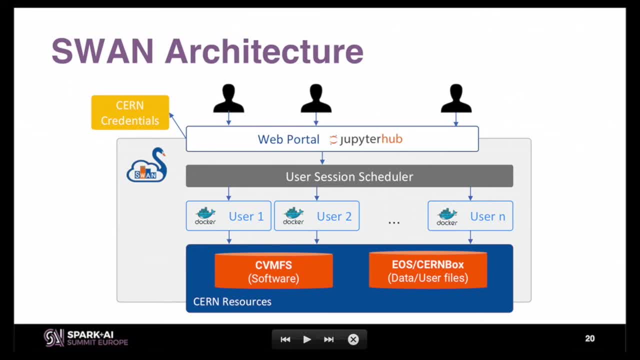 So, as a user, I connect to this web portal Where I authenticate, And then I'm given a session And inside this session, I have accessible all the software that I need from CVMFS And all the data that I need. 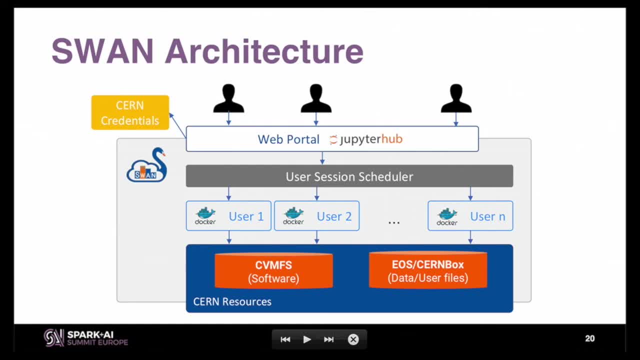 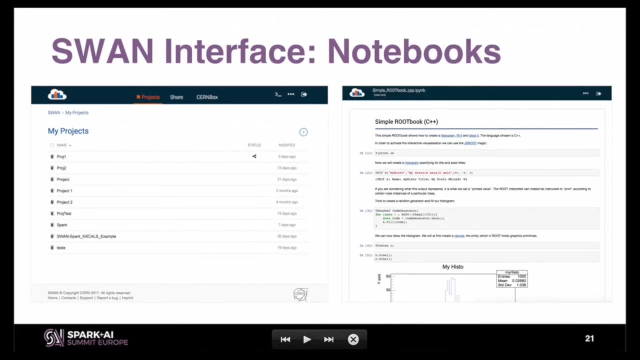 Collision data that is stored on EOS or on my private space, on my CERN box, Which is actually my home directory in this service. Then the interface is the notebooks. I guess you are more or less familiar with it. So it's this interactive computing interface. 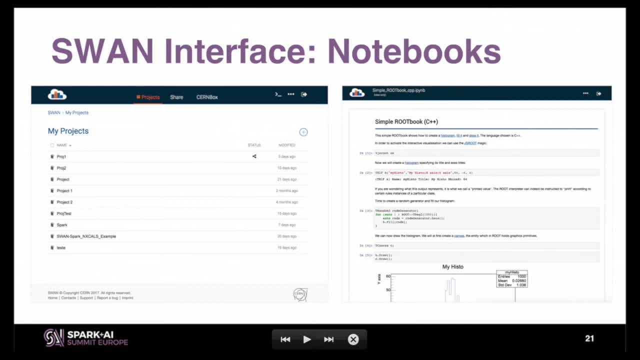 Where you can combine different types of data. You can have text explaining what you are doing, You can have code that you can run And you get back the results, Which can be text or graphics. Everything is in the same document And people can create their notebooks. 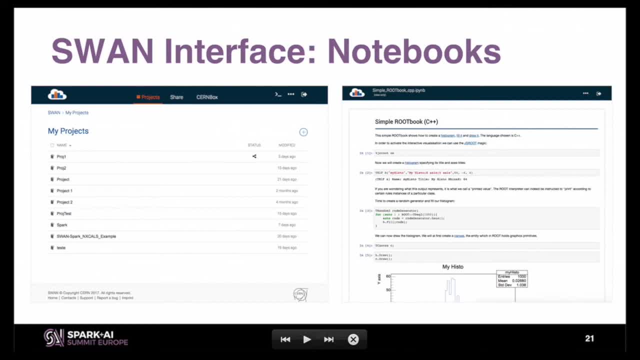 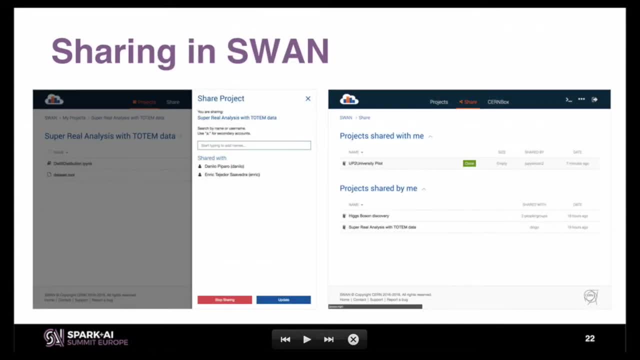 They can create projects that contain these notebooks Plus some input data, Plus maybe output data, And then they can actually share these projects with other people. So from the SWAN interface they can go and they can say: okay, I have this project with. 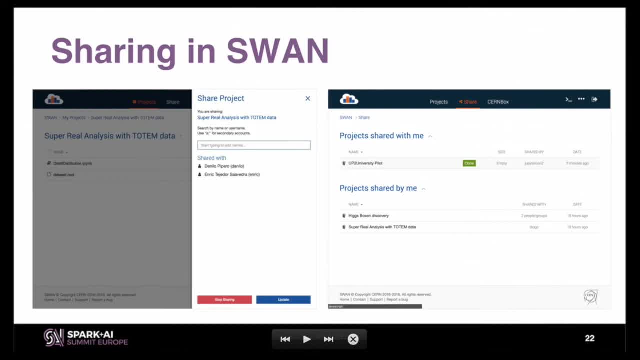 my notebooks. These are the types of data And now I click on it and I want to share it with this guy and this guy And then these other people. they will see it also appearing in their SWAN interface that someone shared this project with them. 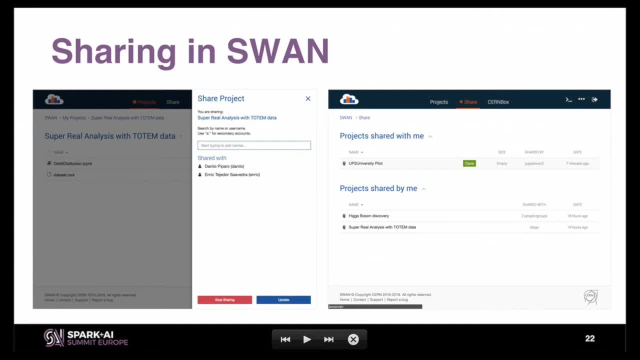 They will be able to click on it, inspect the notebooks, maybe rerun them, modify them and reshare them again if they want. So it really enables this collaborative analysis that we really need at CERN. And then the last ingredient of this platform is actually the integration with the database. 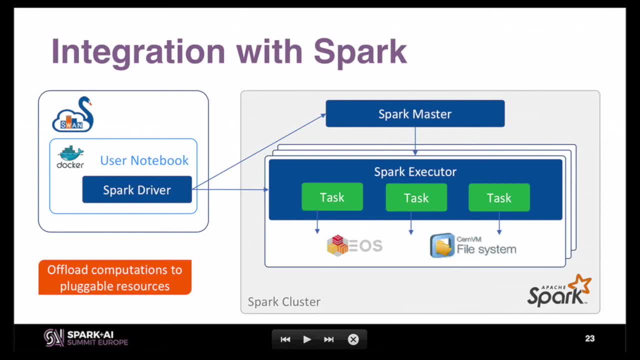 So this is the integration with the database. This is the integration with the database. This is the integration with the database. This is the integration with Spark, Because we didn't want that our users were restricted to only the resources of their session, which is actually encapsulated in a Docker container. 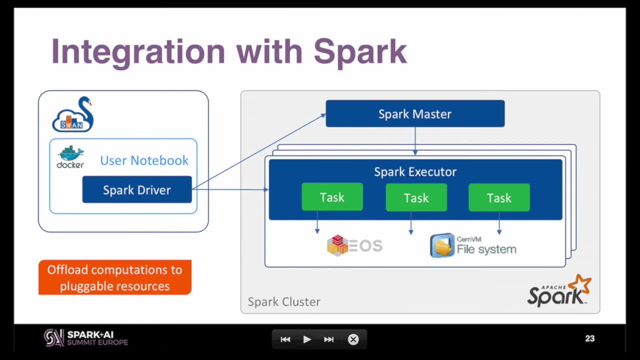 We wanted them to be able to go beyond these resources and to spawn computations elsewhere, to an external cluster, And we actually started doing this with Spark. So now in SWAN, since the beginning of this year in production, we allow users from a notebook to submit their resources. 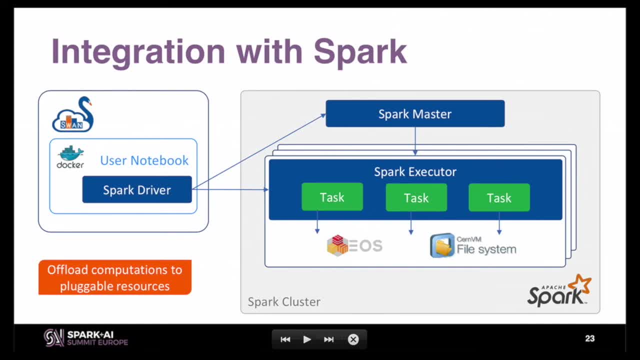 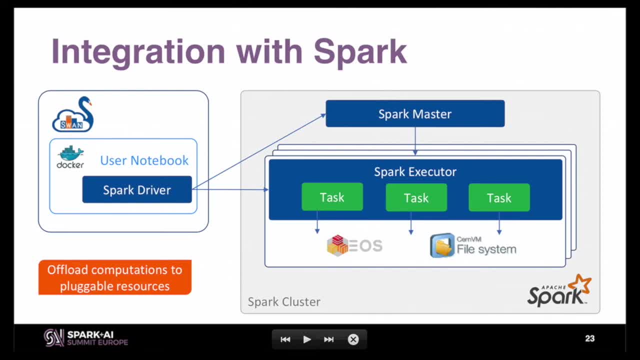 And, of course, these tasks. they will also have access to the data on EOS and to the software that is installed on CBMFS right, Because we really want to replicate the same environment, let's say on the client side, in my notebook and on the Spark executors. 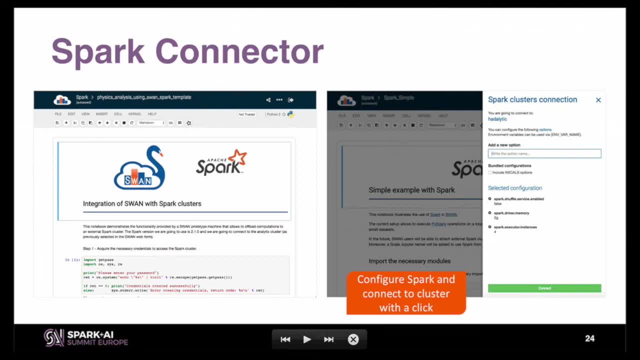 So what users typically do when they want to use Spark, They go to SWAN. They have this interface to connect to a Spark cluster. They can also provide some configuration like number of executors, memory per executor, et cetera. 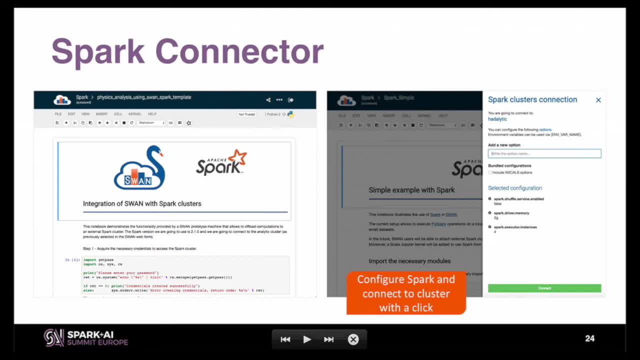 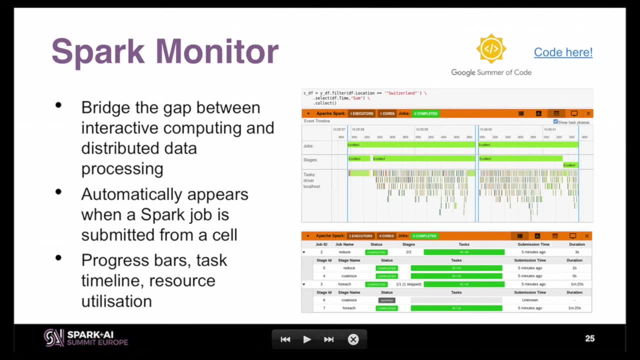 And when they are happy with this they click on connect So they can connect to this particular cluster. And once they are connected they can already from their notebook they can already submit Spark jobs, Like you see in this picture, And when you do that from SWAN automatically in the output of the cell of the notebook. 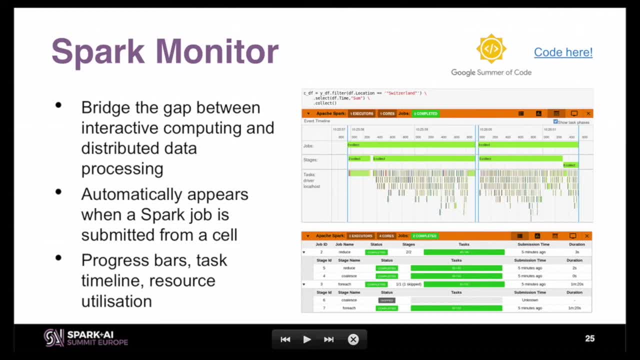 you will see this display appearing. It's an interactive JavaScript display that shows you the progress of your jobs, that shows your tasks where they are running and, if they failed, why they failed, So you can do debugging with it. And actually this was very important for our users, because here you are kind of mixing. 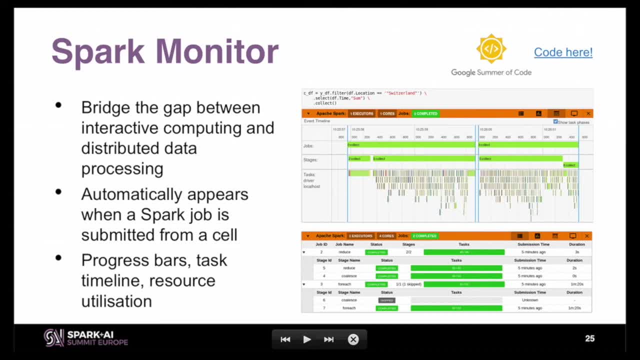 two different environments. You are mixing Jupyter notebooks, which is something interactive. So Whenever I run, I type something on my notebook. I expect that immediately I get a result. You are mixing this with an Apache Spark job that can take some time to run. 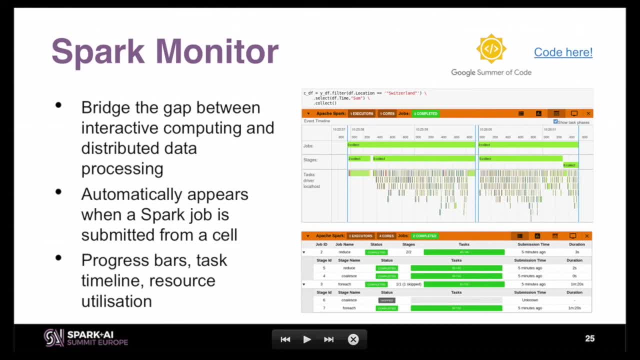 So you really need to provide some means for the user to really know what's going on on the other side, And this is what we do with this display. Actually, it's a. It was in the scope of a Google Summer of Code project. 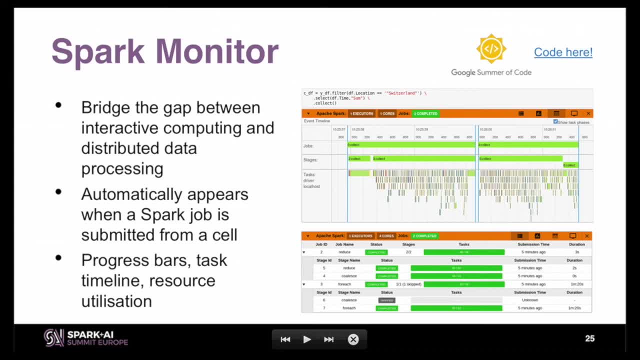 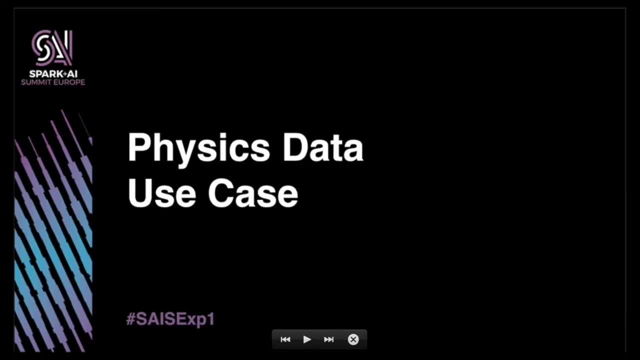 So it's open source. You can download the code of this Spark monitor if you are interested. It's available. So, after describing this swan service, how it combines storage and software at CERN with processing power, with Spark, now I'm going to explain a couple of use cases that are: 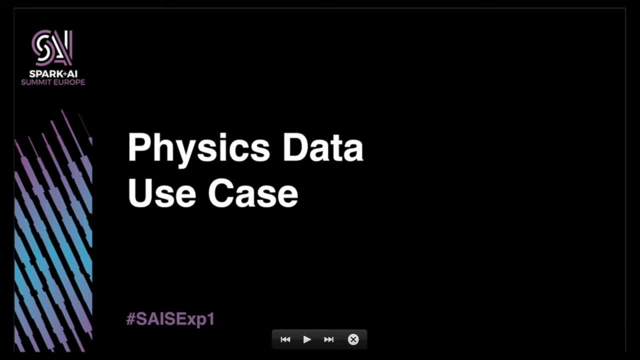 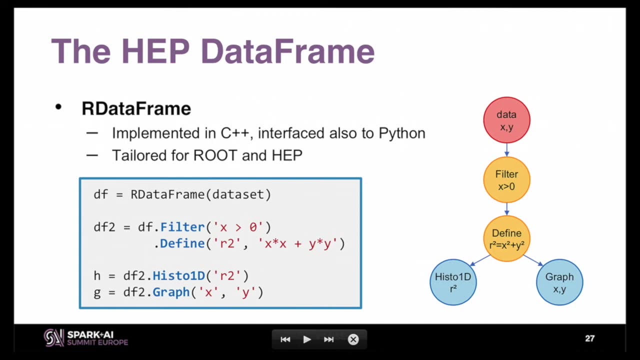 already using this service. The first use case is about analyzing physics data, so collision data coming out from the LHC, And first I wanted to talk about this R data frame that we have. So in root we have our own data frame. 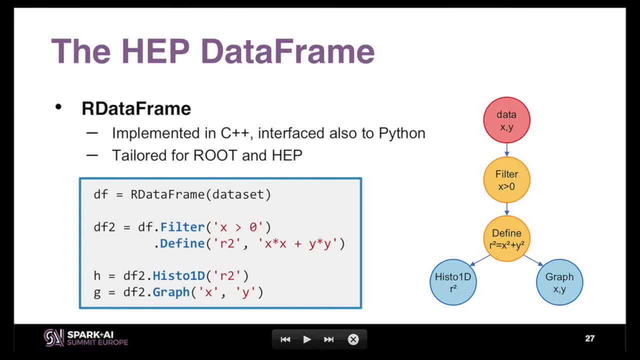 It's called R data frame And in a way it's similar to the Spark data frame. So it promotes this high-level declarative analysis model where you express your computation in terms of operations on a given data set. So you can see in this small code example how some operations might be familiar to you. 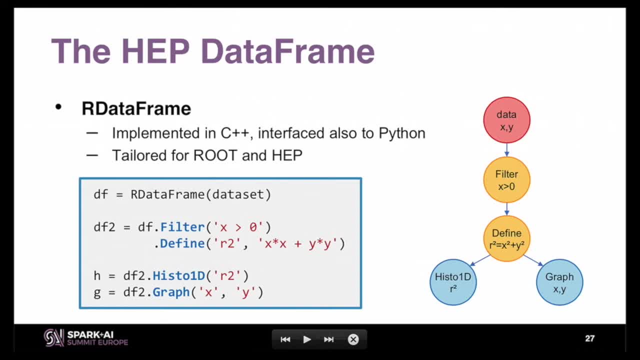 Like. you can define filters on your data, You can add new columns to your data set. These are typical operations you can also do in Spark, But there are some operations that they are specifically tailored for our use case. Like typically physicists, they want to make sense of the collision data. 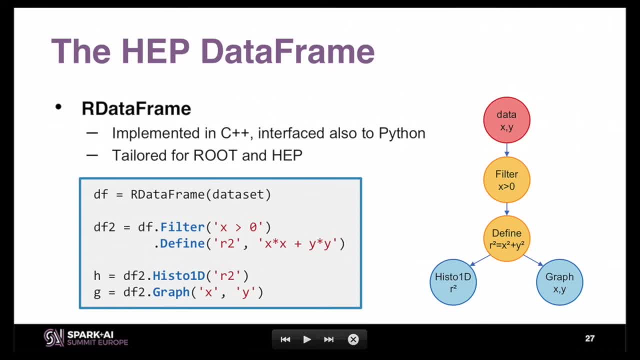 They create histograms or graphs, And these are actually actions that we have in our R data frame that generate these entities that then physicists they will use in their analysis. And another cool thing that you can see here: This is the R data frame. 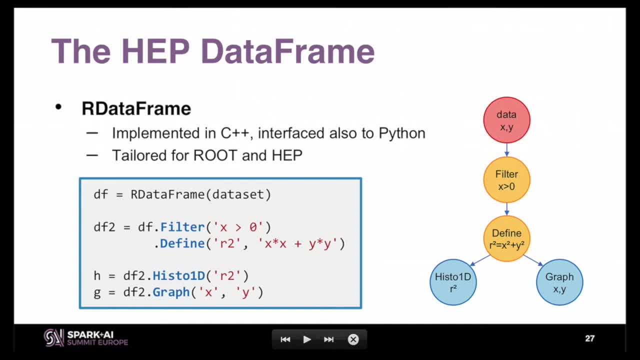 You can see here, actually this is Python code, But the strings that you pass to the filter or define, actually this is C++, Because R data frame and root, they are implemented in C++. So Python is only the interface. We have an interface for Python users. 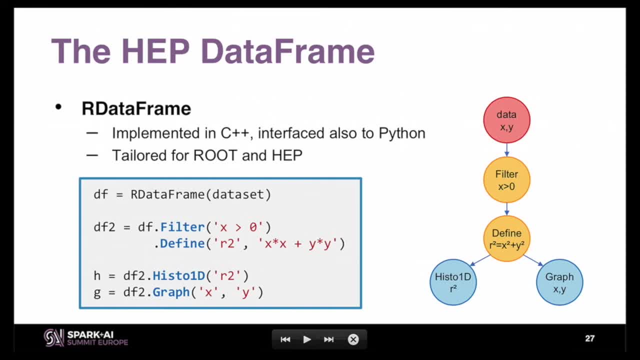 But here what we do is root has a C++ interpreter, which is called cling. that is actually linked to LLVM and Clang, a compiler, And it is able to take this string, this expression, Basically wrap it in a function and, just in time, compile it and run it. 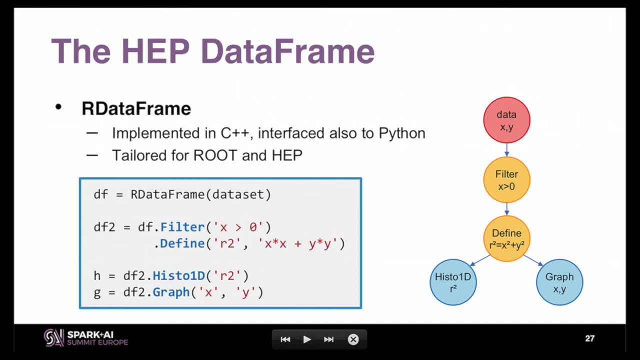 And in this case it's a trivial cut, but it could be a more complex cut, like in the case of physics. we have functions with many lines of code that define our cuts right, So we could actually also do this from here. 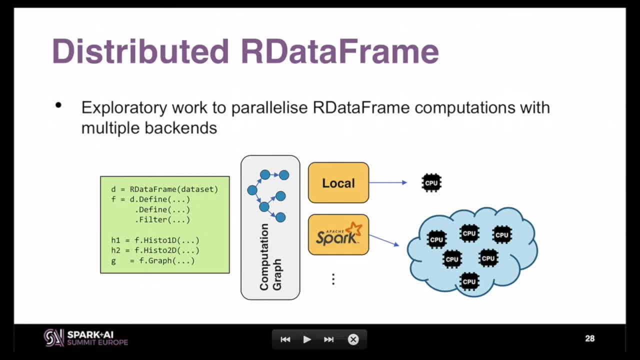 Then with this R data frame we wanted to exploit Spark R data frame. now it can run on a single computer, also exploiting all the cores of that computer, multi-thread parallelization implicitly. But we wanted that an R data frame application and R data frame analysis would be able also. 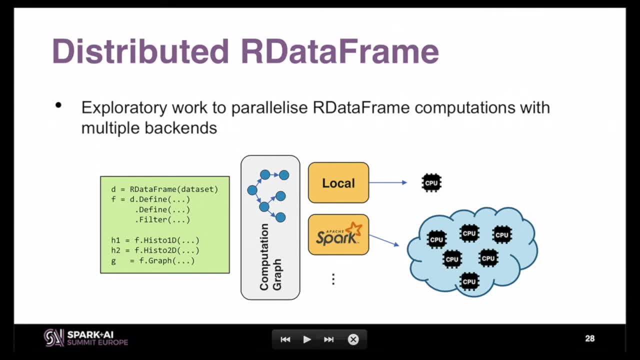 to exploit all the nodes in a cluster and, in particular, the Spark clusters that we have at CERN. So what we did is we developed a backend for Spark in R data frame that is able to distribute this computation graph that is generated by R data frame to all the nodes of the cluster. 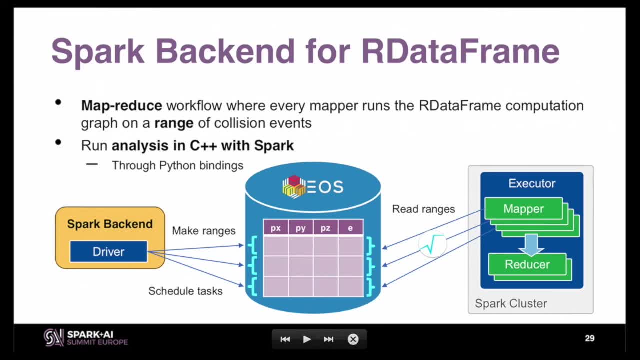 Okay, So you can see how it works underneath. So the Spark backend: it knows the data set you are working on and it will basically divide it in ranges and it will create, with Spark, a MapReduce workflow where the mappers 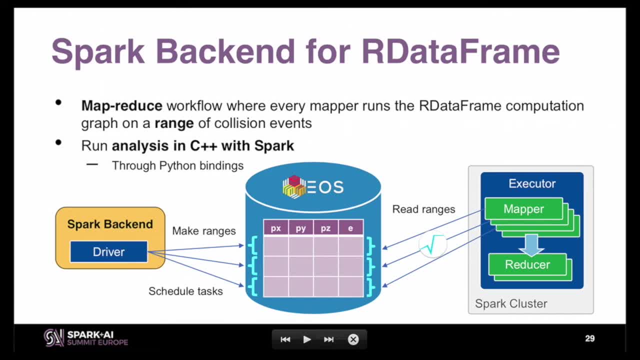 they will use the root IO libraries to remotely read data from the EOS storage system, which is where our data is. So every mapper will read a range with root and then it will apply the computation graph of our data frame. It will generate some results, histograms, et cetera, and then this will be reduced into. 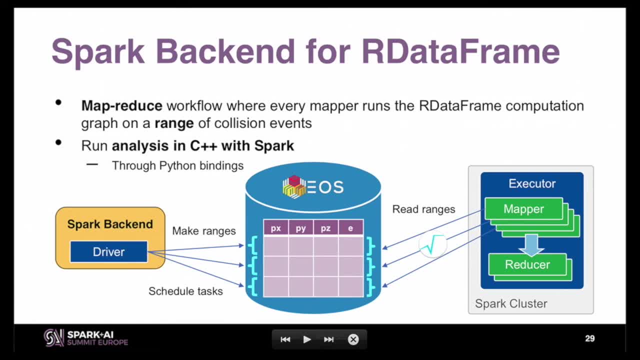 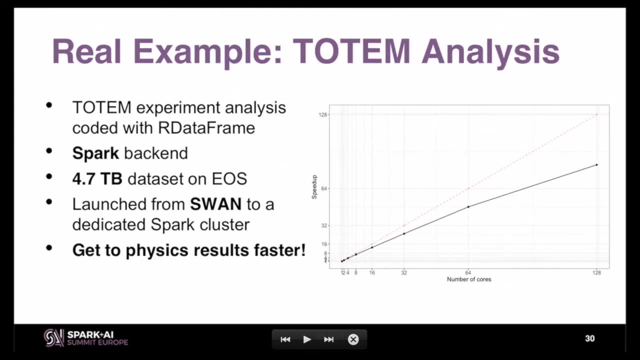 a final result, And here I just wanted to highlight that we are able, with this system, to run analysis that are coded in C++ with Spark, through Python bindings, so through PyRoot and PySpark as well. So we actually, very recently we tried this on. 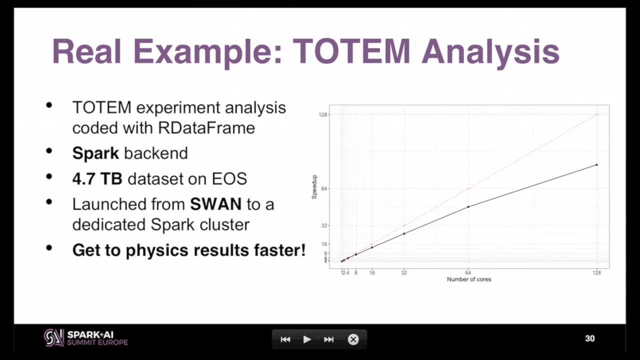 On a real analysis code coming from a CERN experiment that is called Totem. So Totem is an LHC experiment. What we did is we took a code that they had, that they used in their grid jobs and batch jobs, and we converted it to the R data frame form. so this declarative analysis model. 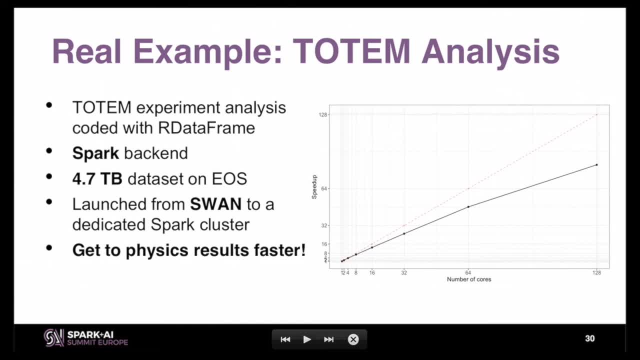 and then we run it with the Spark backend In the. Actually, the input data set was a 4.17.. Okay, So this is the 4.17 terabyte that was stored on EOS and this is collision data from the Totem experiment, real data that they used to actually publish a paper before. 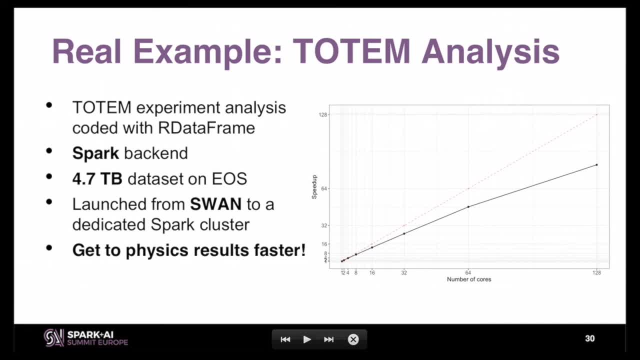 And we launched it from so on from a notebook to a dedicated Spark cluster that we had. And this is the scaling, the preliminary results of scaling, that we got Here. actually, the application is basically IO bound, so there's not a lot of computation. 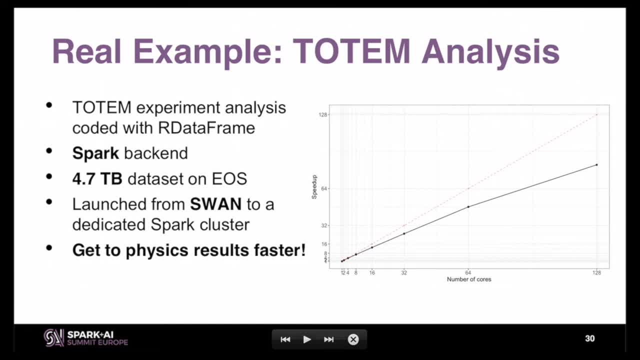 going on in the mappers, because we are basically filling histograms. Okay, So clearly the- Actually the resource utilization could be improved. but the point that I wanted to make here, which I think is important, is that for the maximum number of resources that we 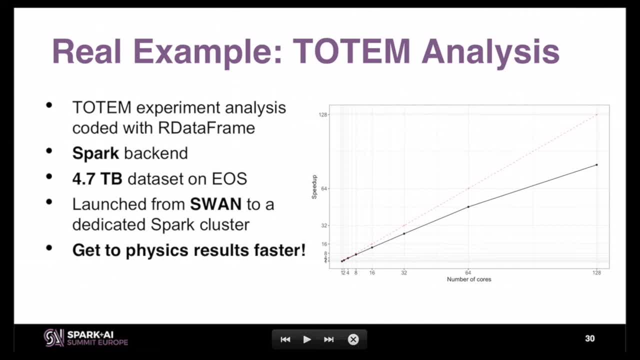 were using here, their analysis run on the entire data set in a few minutes And when the same Totem colleagues they run these with batch or grid jobs. it normally took for them from several to many hours to run the thing on the entire data set. 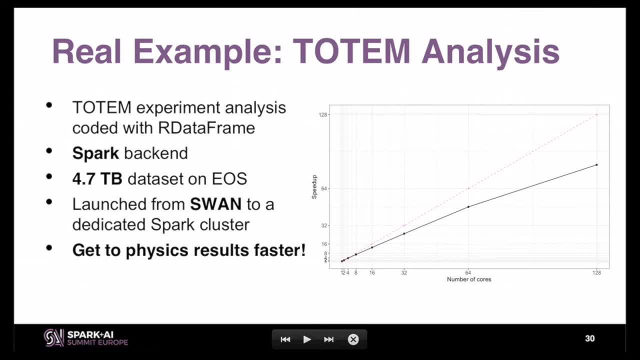 And although we cannot compare it because these are different infrastructures, we can't compare it. This is a Spark dedicated cluster and the other one is the grid For physicists. it's important. So physicists, they are interested in physics, right. 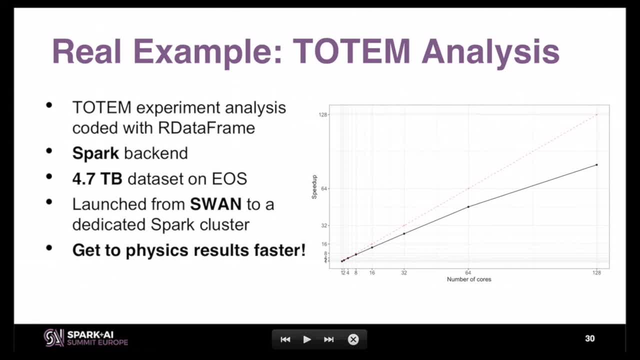 This is no surprise. So whatever system brings them to physics results faster, it's more likely that they will adopt it, that they will change the way they do things to adopt this new thing, And I think these results, although they can be improved, they are encouraging these people. 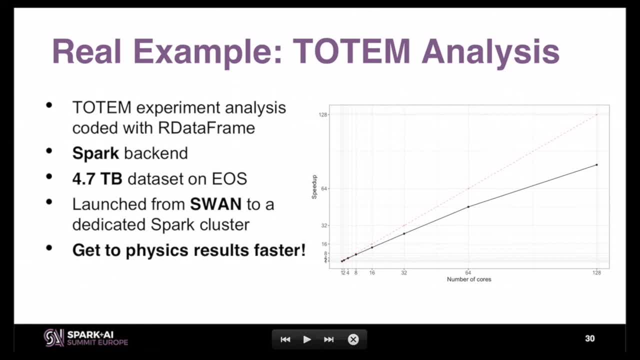 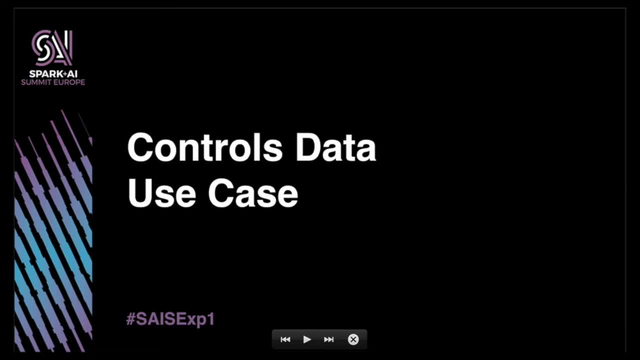 to continue exploring the Spark way. Okay, So now I'm going to. Before finishing my presentation, I'm going to talk about another use case. that is, exploiting the SWAN service at CERN to run with Spark. So this is not physics data anymore. this is not collision data, this is actually log. 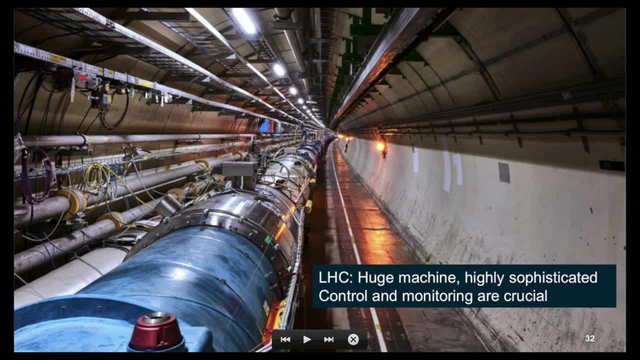 data Controls- data that comes from the LHC, because the LHC is a highly sophisticated machine, so when it's on operation you really need to know what's going on. You need to control with a lot of devices that are installed in this LHC different. 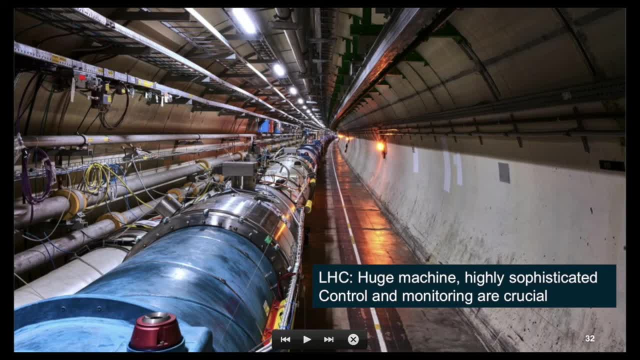 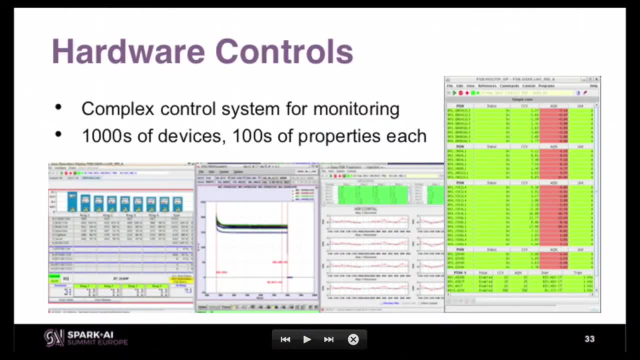 parameters to understand if everything is going well or not. Actually, there's a whole team of people dedicated to that to operate the machine, and what they have is they have thousands of devices installed on the LHC with hundreds of properties each I don't know: temperatures, pressures, properties of the proton beams, many, many things that 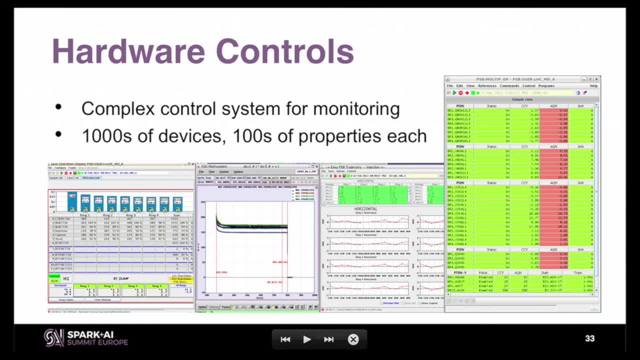 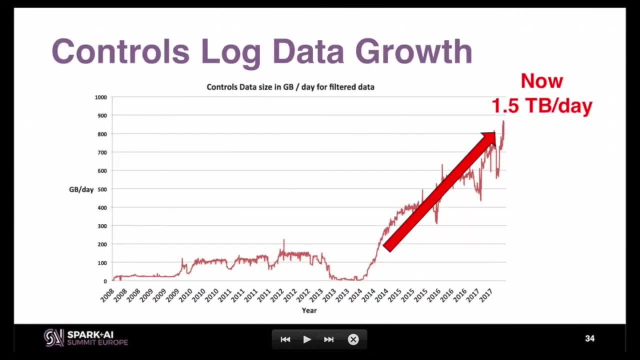 they need to control and that they need to monitor. So they actually log all these things, all the information from the devices, and they actually recently they started even logging more devices and they increased the frequency at which they log and they saw this kind of explosion in the volume of data that they 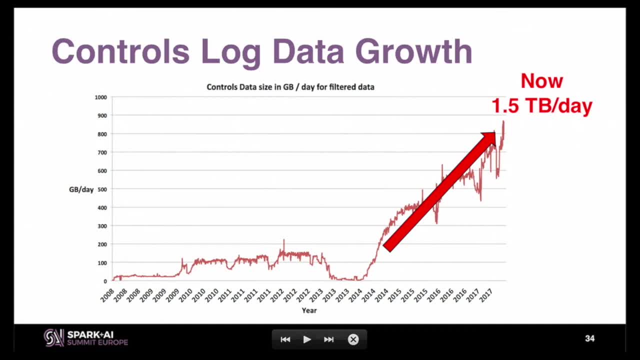 need to store. Actually, now they are storing 1.5 terabyte a day. That's the data of logging data that comes from the LHC, And this made them realize that their current system that they use to analyze this data was not usable anymore. 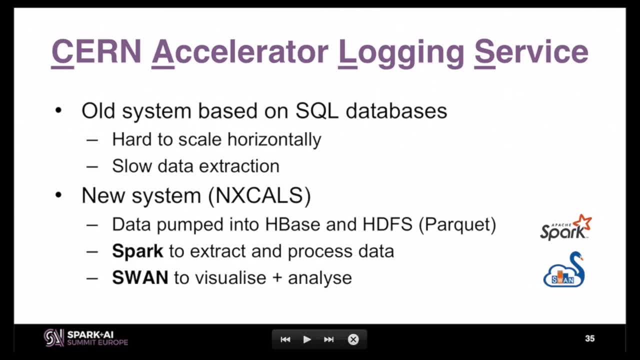 They had this system based on SQL databases that was not scaling anymore. It was slow for them to extract data from this system and analyze it. So they are actually moving already now. So actually for this team of people, the problem is already here. 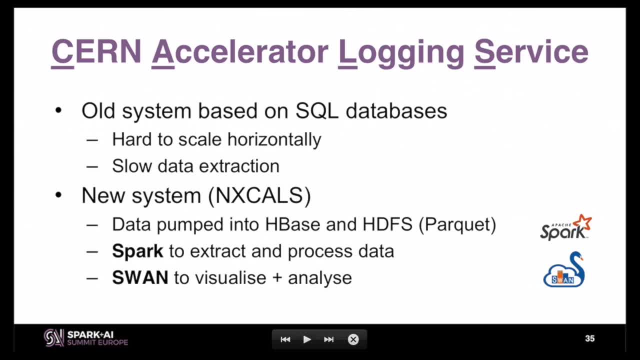 I talked about the physics data before And I talked about This is 2025. But these people have the problem now and they are already moving to a system where they don't dump the data on SQL databases anymore. They pump the data into HBase and HDFS. 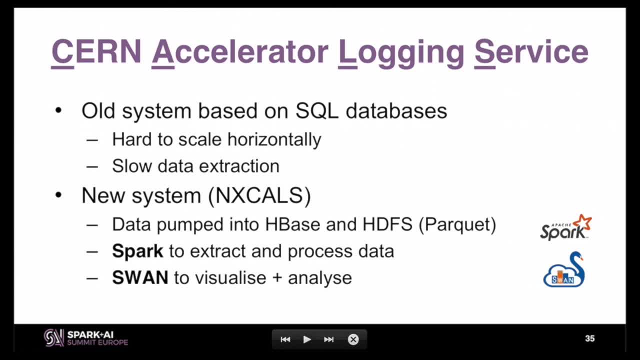 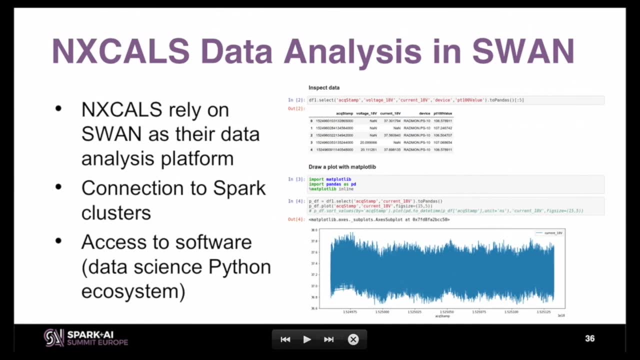 And on top they use Spark to extract and process that data And, in addition, they do this from SWAN. So SWAN is the entry point for these people to process their log data And they are On a daily basis. they are producing these notebooks where they use Spark to query their 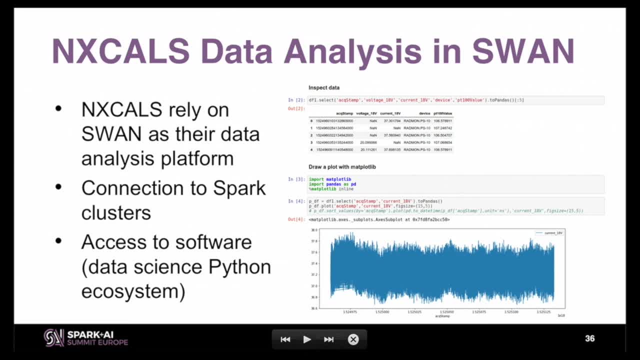 data or to process their data. They get back some results. They use the software that is installed on SWAN in order to analyze this data And they produce these notebooks that they can share between each other. So they really rely on SWAN as the entry point to accessing these Spark resources. 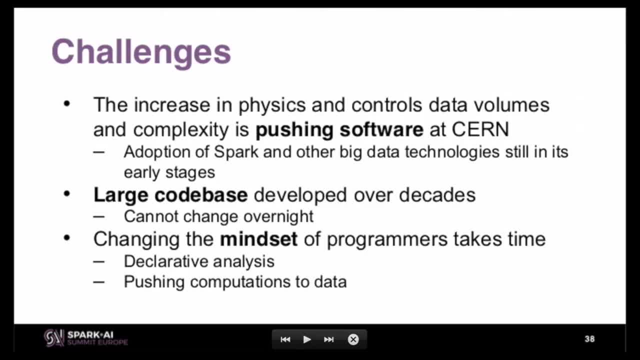 So I come to the end of my presentation, Just as a summary, Okay, Okay. So I have already mentioned all these challenges that we have ahead at CERN. We are seeing how we will have in the future this increase in physics data. 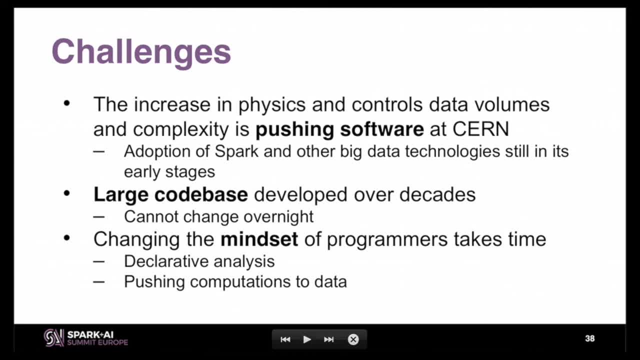 We already have an increase in controls data And this is pushing software at CERN a lot. So we are looking, of course, outside and seeing what other people do, what is used in industry in the big data field, But I would say that 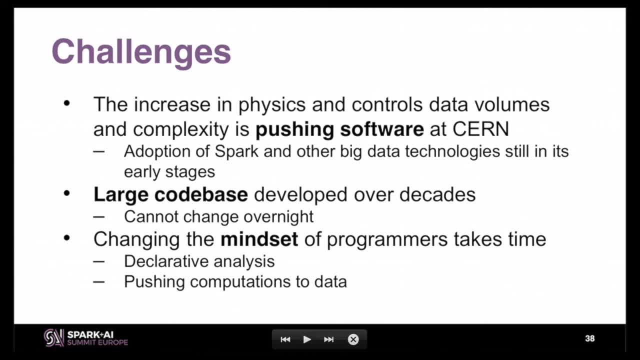 The adoption of Spark and other technologies coming from big data. it's still in early stages because in the end, we have all these traditional ways of running our code that have been very successful And we have a large code base of experiment software that does things in a given way. 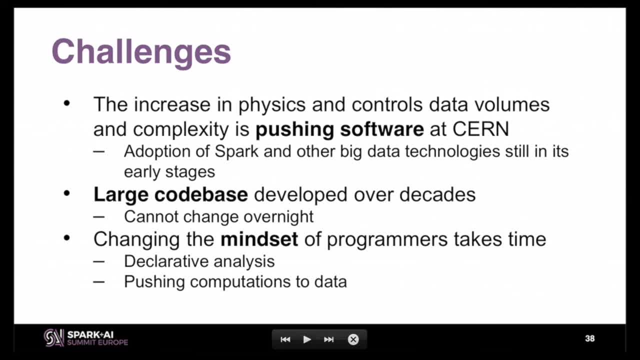 So this, of course, cannot change overnight, And it's not only the code, It's also programmers- Programmers that are used to programming away Physicists, And it's difficult to change the mindset that they have like promote these higher-level. 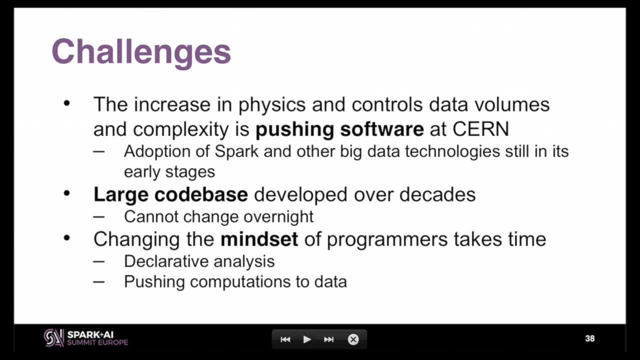 programming models. So now you are going to express your analysis with data frame style, instead of just doing an explicit loop on your collision events Or pushing computations to data. Instead of getting all your data to your machine and then analyzing it in your machine, you 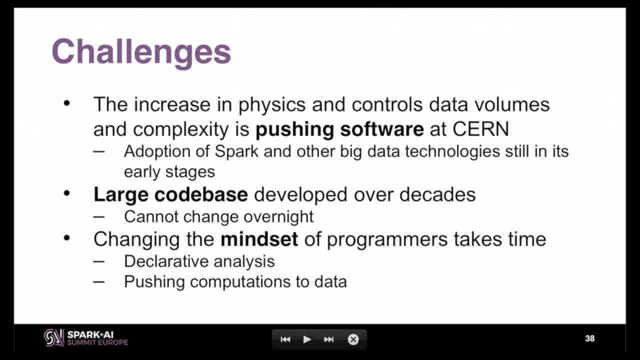 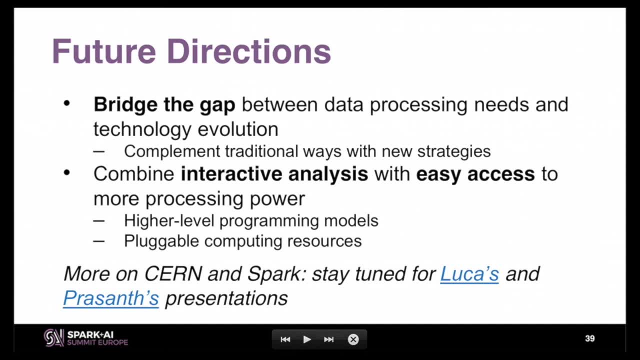 need to try to push computations to data. This all takes time to adopt, Right, But we know that we need to bridge this gap between what will be the technology evolution and our data processing needs, And we are working on that And this is why we are going ahead with this project, with this SWAN service to combine. 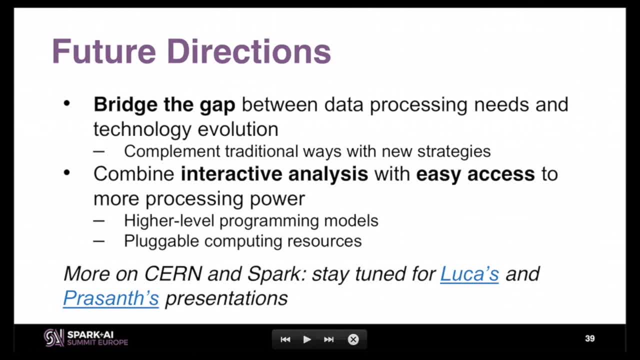 interactive analysis with a nice interface, where people can easily offload computations to external resources to plug these resources and use them to run their analysis, And where we promote these higher-level programming models. This is all I wanted to say, Just to finish with. 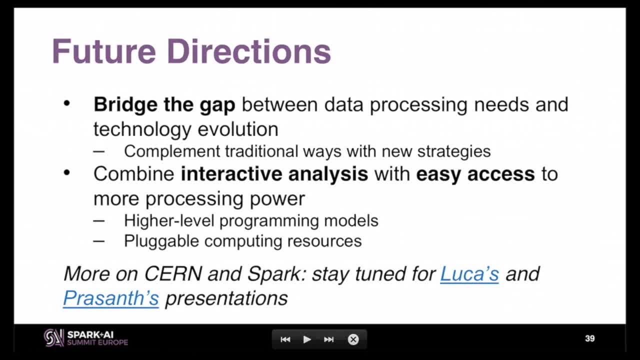 There will be a couple more presentations by Luca and Prashant about CERN and SPARC, So if you are interested, stay tuned. Thank you, You mentioned that SWAN has the capabilities to share notebooks and all this. Yes, Could you give some more details about this function? 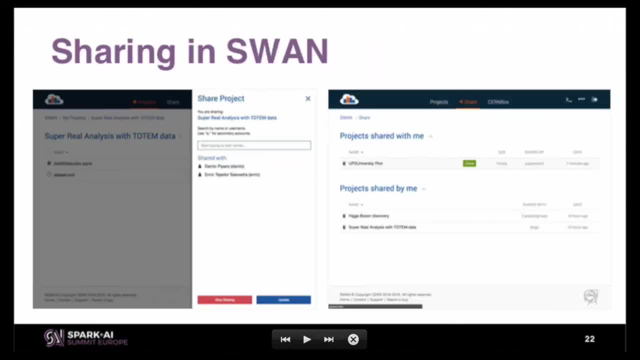 Sure, Let me go back. Yes, So the idea is that SWAN has a home directory. So when you log into SWAN, your home directory is your CERN box, where all your files are, And CERN box has the capability of sharing. 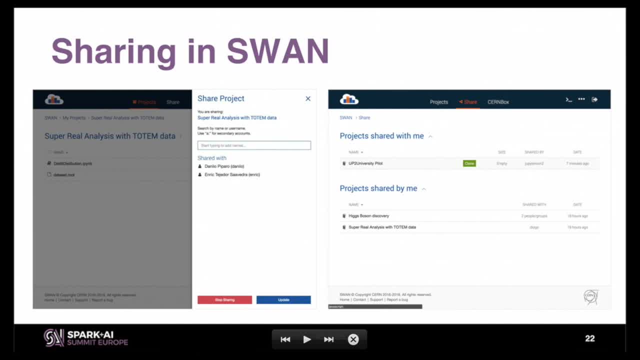 It provides sharing primitives. So what SWAN does is actually uses an API of SWAN, So you can go and say: okay, so this project, which is actually a folder that contains notebooks and other types of data, I want to share it with these people. 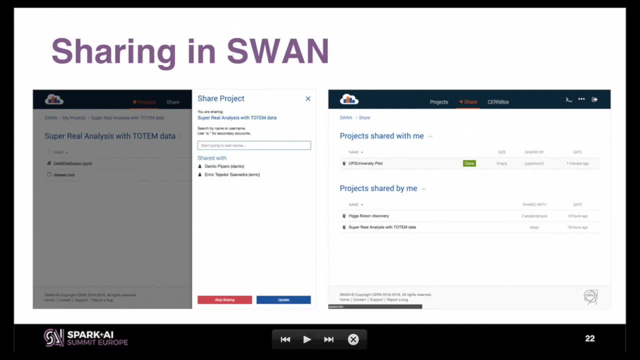 And then these people, they will see it thanks to CERN box. they will see it appearing also on their SWAN. And another thing that you can do with CERN box is it's a little bit like Dropbox, So you can install a client in your laptop and you can synchronize the files from the